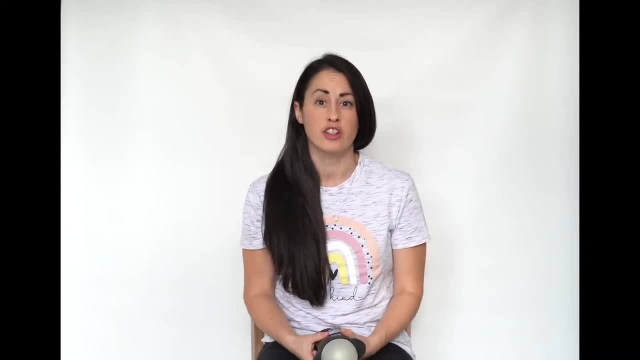 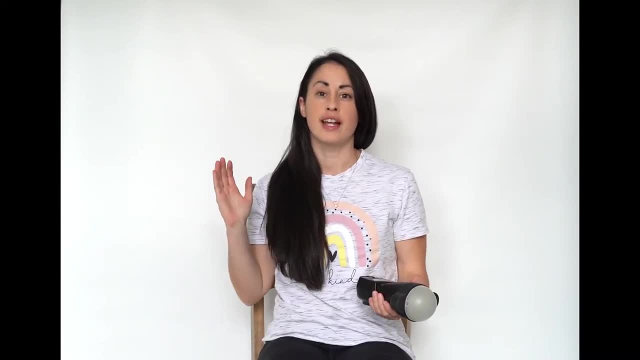 number one factor, and there's lots of different type of lighting that you can use. you can use something called backlighting, and I love to use that during sunsets, where the sun is kind of setting behind your subject, kind of giving off this beautiful glow you can use. 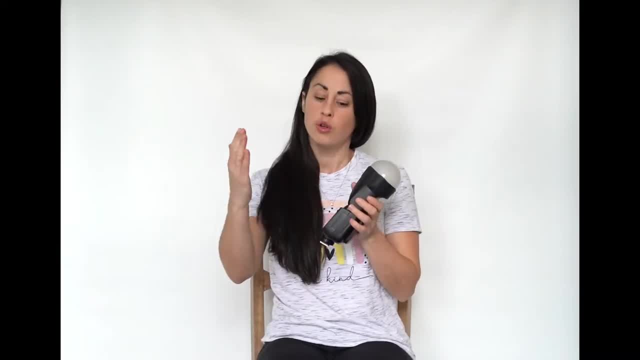 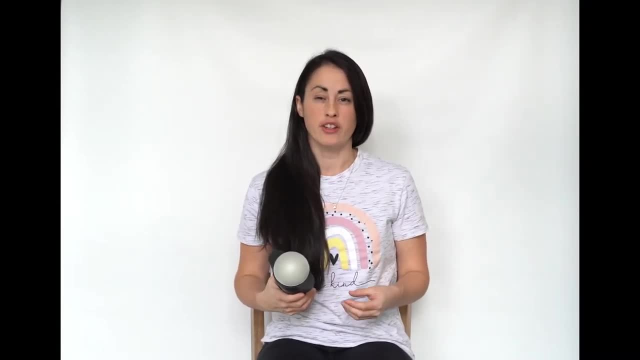 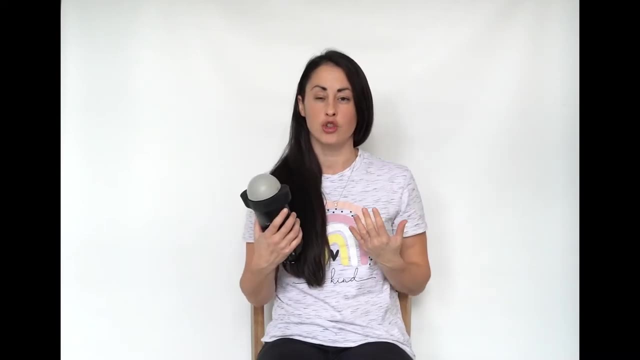 catch lights and that's when you face your subject towards the light and it kind of brings a little bit of sparkle to their eyes. um, you can use low lighting to create dramatic depth and shadows. you can use window lighting or natural light, and I'm actually using natural light right now to 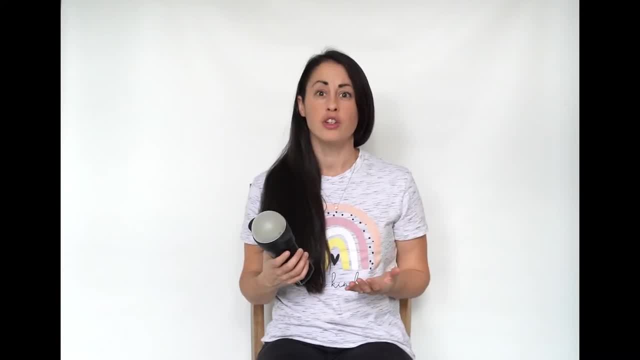 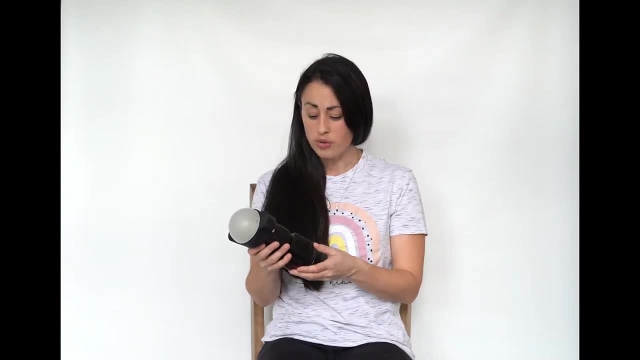 create this video, and if you don't have enough light, you can even use something called artificial light, where you're creating your own light using a tool called a flash, and all you really have to do is you just pop this on top of your camera, and when you need a little bit of extra light, 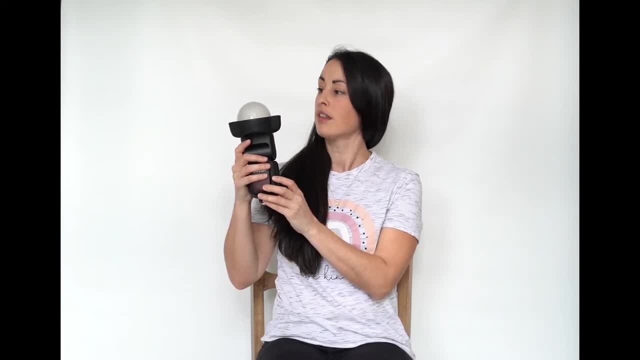 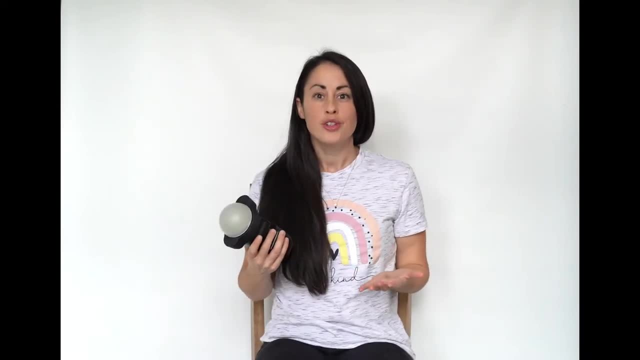 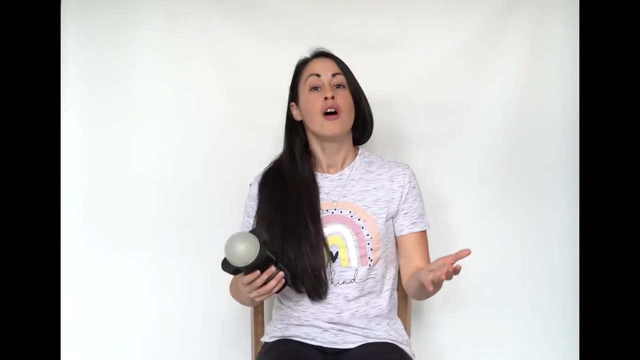 it kind of goes off just like that. there we go. now, if you don't have a flash- and a lot of people don't, and that's okay- you can use the flashlight, because that's what my kids like to use when they need a little extra light in their pictures too. um, so follow along with me, we're going to go. 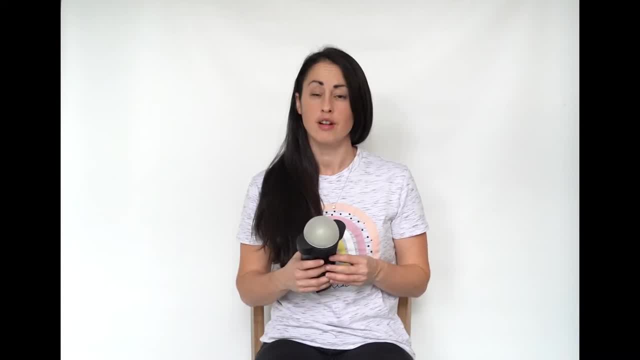 through each one of these, and then we're going to go through each one of these and we're going to go through each one of those different lighting examples that I just talked about, and I'm even going to show you some examples of what that lighting actually looks like and how it can. 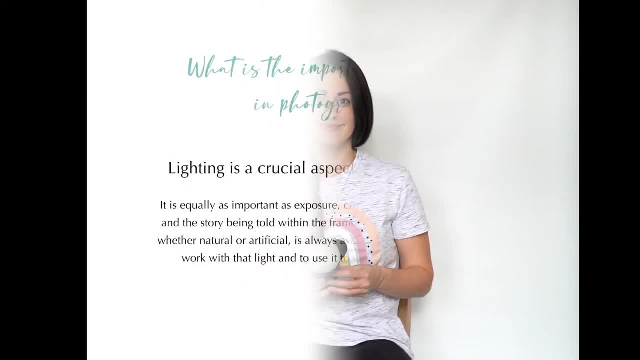 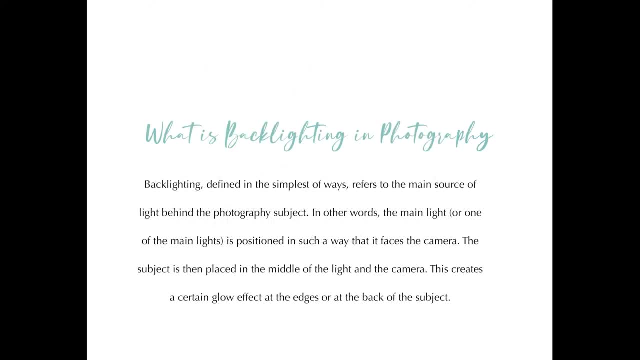 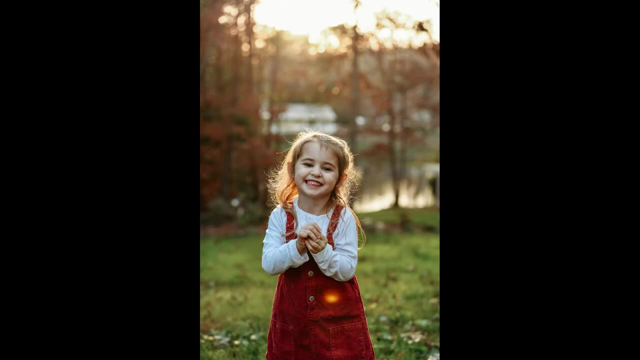 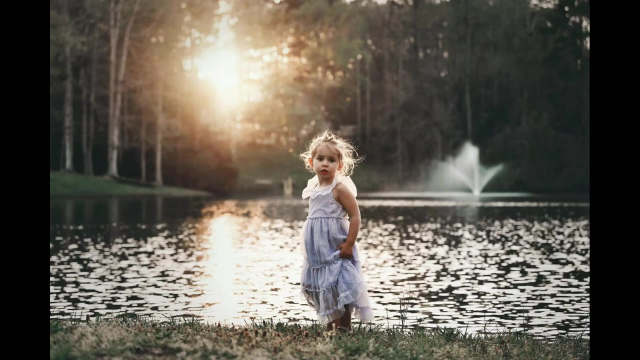 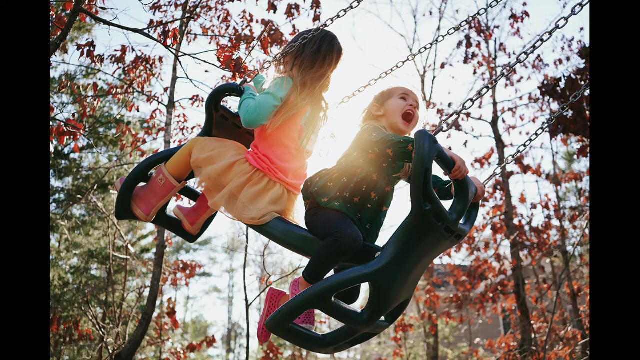 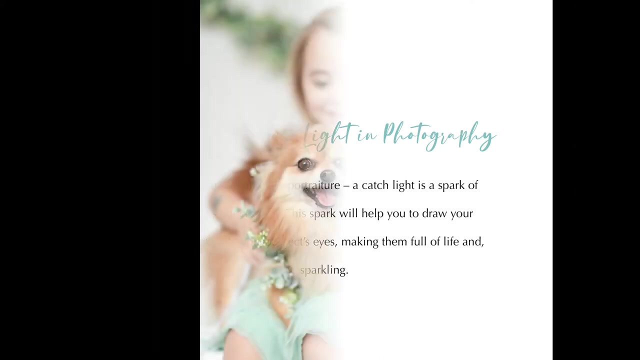 change your pictures. light is essential to photography. understanding and paying attention to all the different types of light can help you improve your photography skills. you have back lighting, and that is when you place your subject in front of the sun to give this nice warm. you have catch lights, and that's when you place your light source in front of your subject to give a